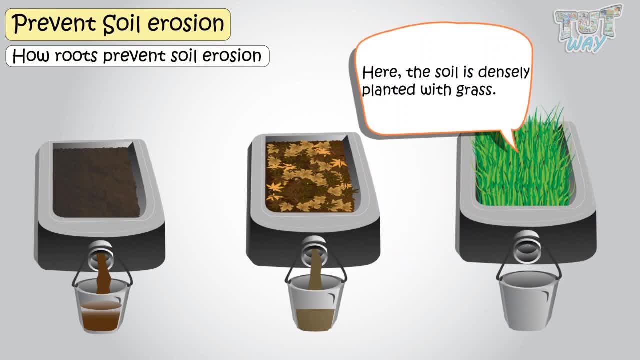 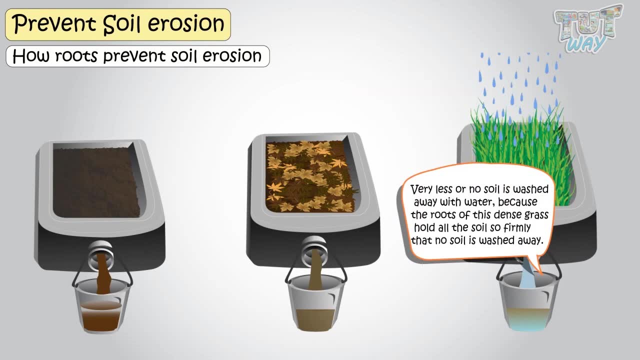 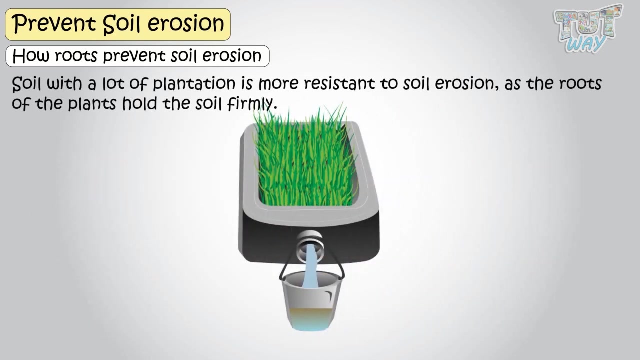 densely planted with grass. Now if you let the water flow above soil in this container, very less or no soil is washed away with the water, because roots of this dense grass holds all the soil so firmly that no soil is washed away. This shows that soil with a lot of plantation holds the soil. 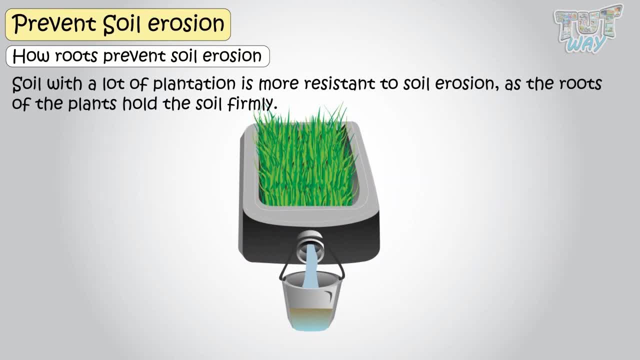 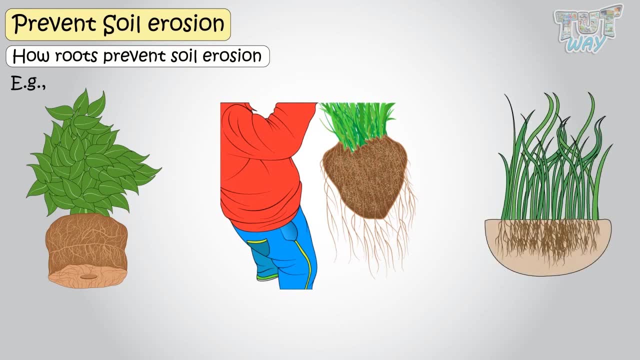 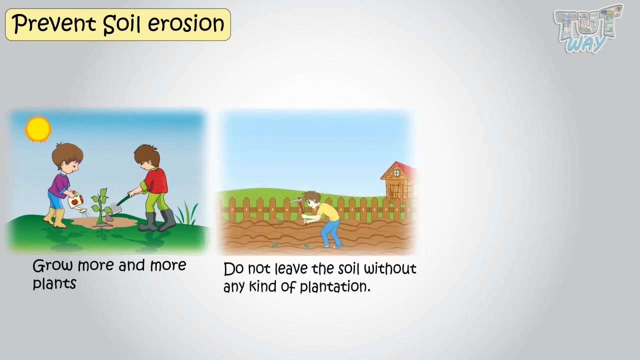 firmly and prevents soil erosion. Let's have a look at more examples. These things show how roots hold the soil together and prevents it from being washed away or prevents soil erosion. So the first thing to prevent soil erosion is: grow more and more plants and do not leave soil without any kind of plantation, and prevent soil erosion. 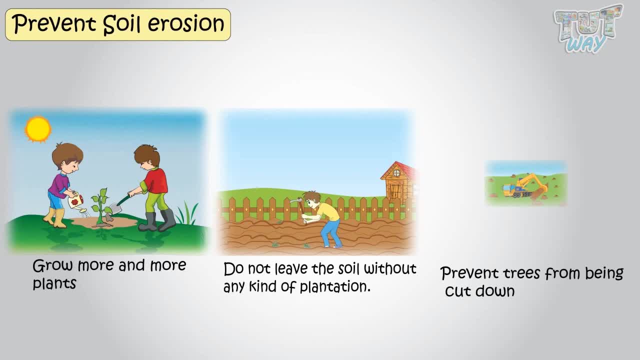 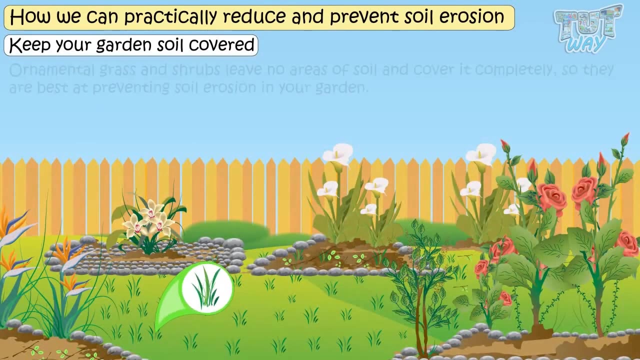 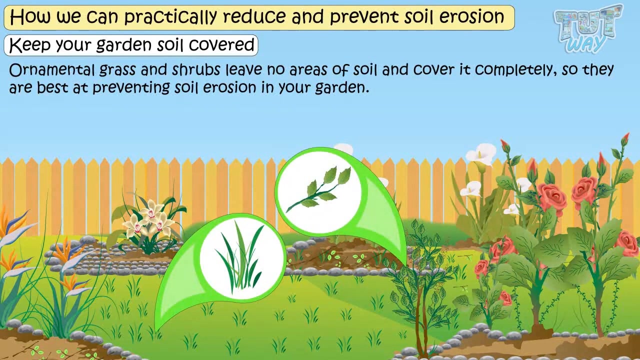 trees from being cut down. Now we know that plants prevent soil erosion. Now let's learn some points: how we can practically reduce and prevent soil erosion. Ornamental grass and shrubs leaves no areas of soil and cover soil completely, so they are best at preventing soil erosion in. 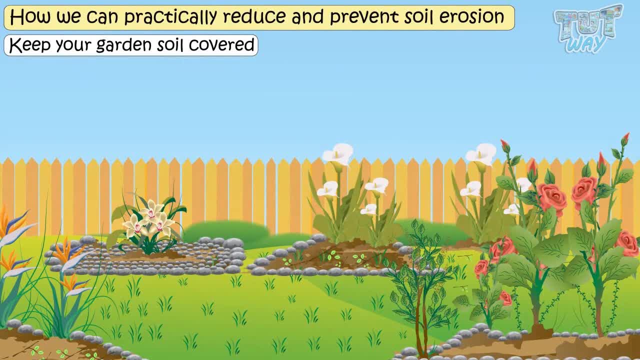 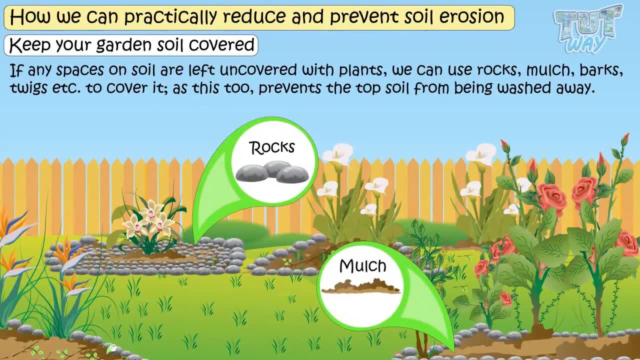 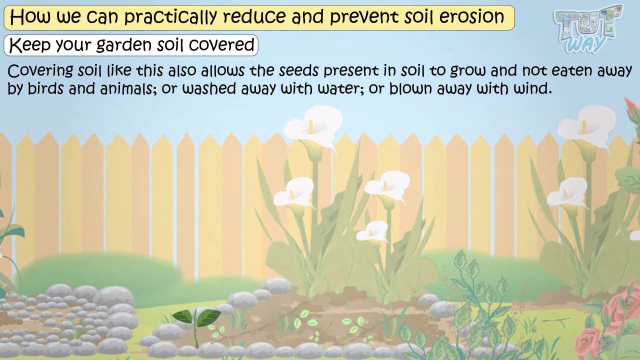 your garden. If any spaces on soil are left uncovered with plants, we can use rocks, mulch twigs to cover it, as it, too, prevents the topsoil from being washed away. Covering soil like this also allows the seeds present in soil to grow and not be eaten away by birds and animals. 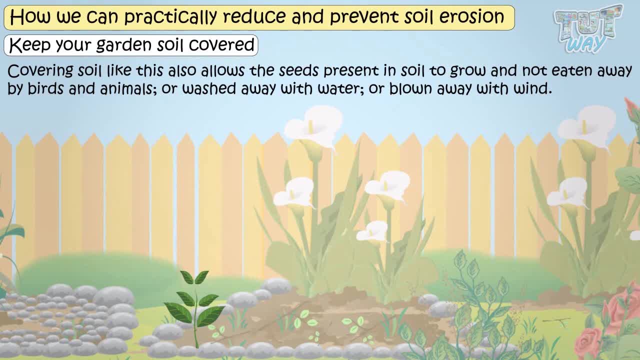 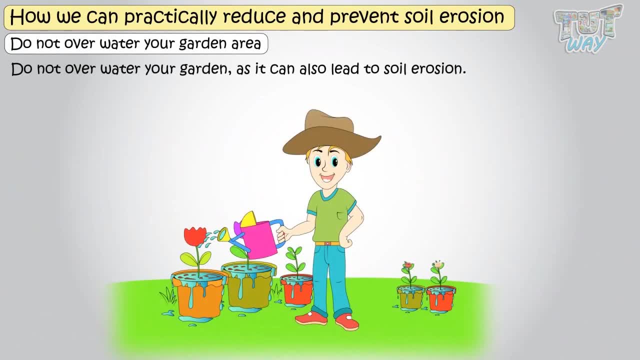 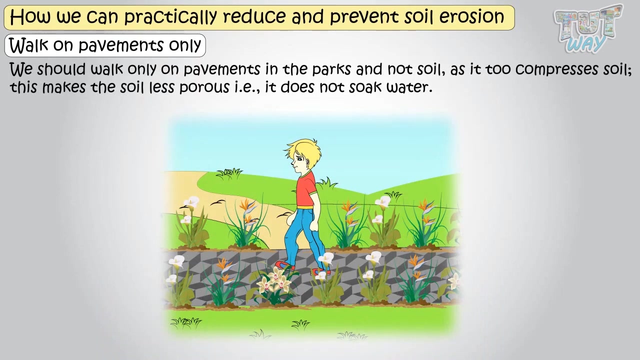 Next is: do not overwater your garden, as it can also lead to soil erosion. We should walk on only pavements in the parks and not soil, as it, too, compresses soil. That makes soil less porous. Next is: it does not soak water, and water runs off from above this soil, along with precious topsoil. 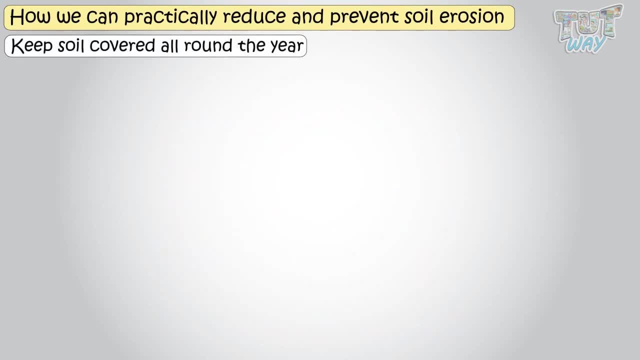 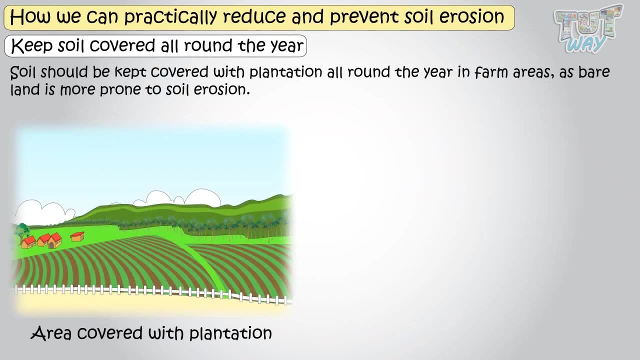 Keep soil covered all round the year. Soil should be kept covered with plantation all round the year in farm areas, as bare land is more prone to soil erosion. Also, keep dizzy and be careful with soil contamination. Do not overwater your garden, since soil is not. enough of an area to be able to absorb soil. The soil should also be kept covered with plantation all around the year in farm areas, as bare land is more prone to soil erosion. Also, don't overwater the grass and the soil. Soil must be kept out in the deep of the garden, The soil of the garden. 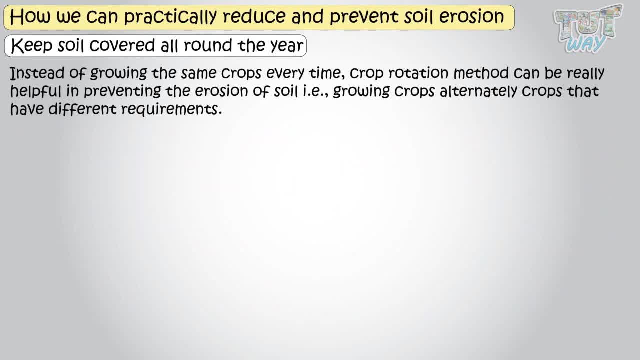 should be kept out in the wet place so it would not be covered by other soil and can be stopped by other soil to get water, And so do not overwater the grass and other soil. Soil shall be kept in a pretty Instead of growing the same crops every time. crop rotation method can be really helpful in preventing erosion of soil. 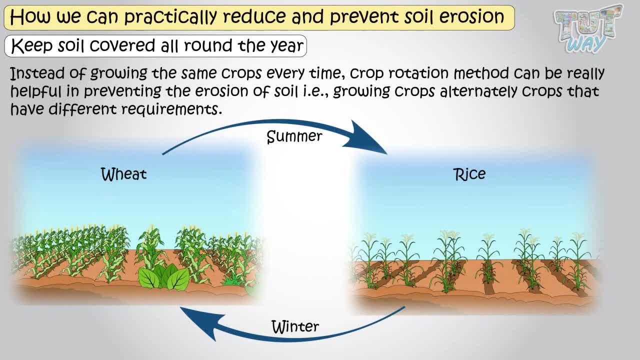 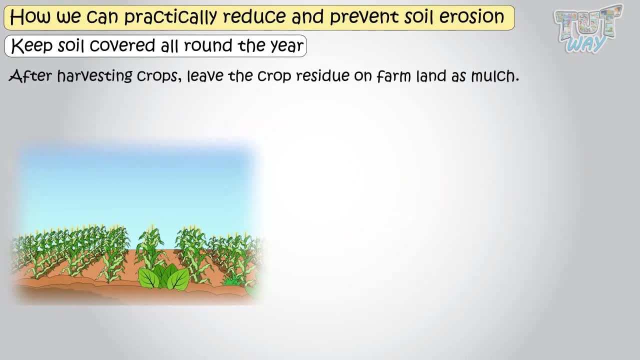 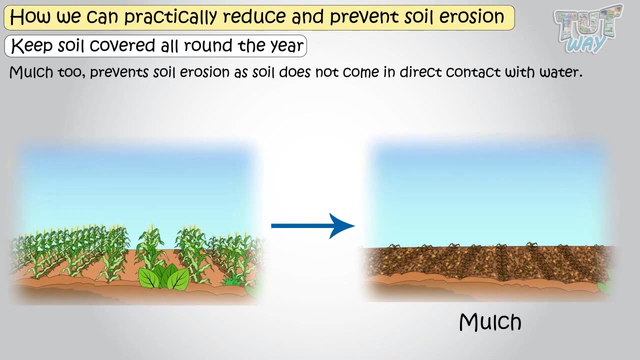 Crop rotation is alternately growing off the crops that have different requirements and, after harvesting crops, leave the crop residue on farmland as mulch, That is, decaying leaves, twigs and bark, which too prevent soil erosion, as soil does not come in direct contact with water. 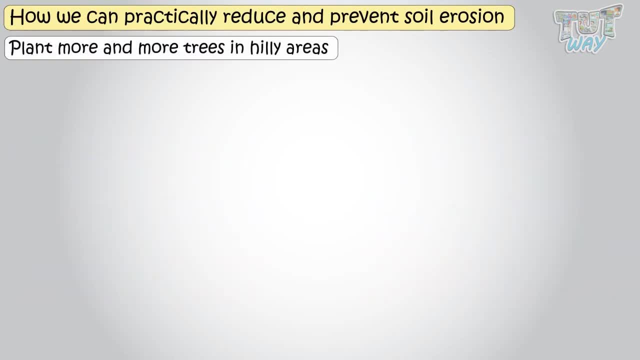 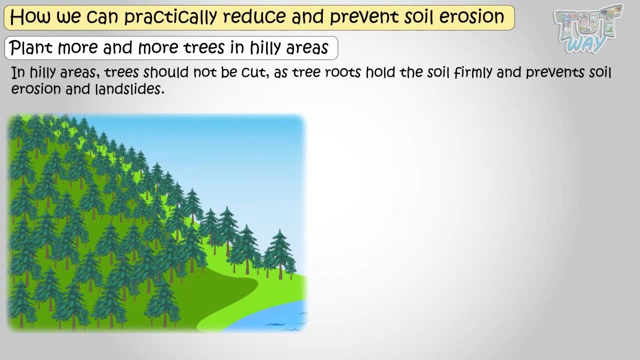 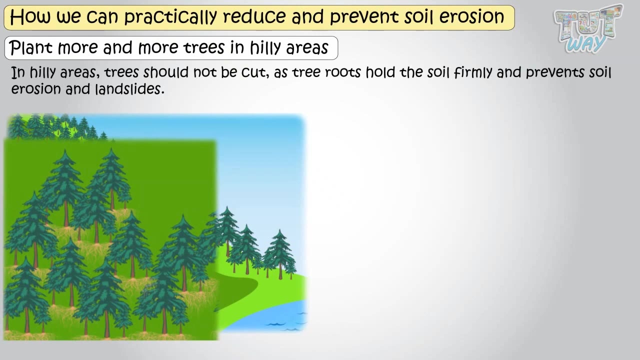 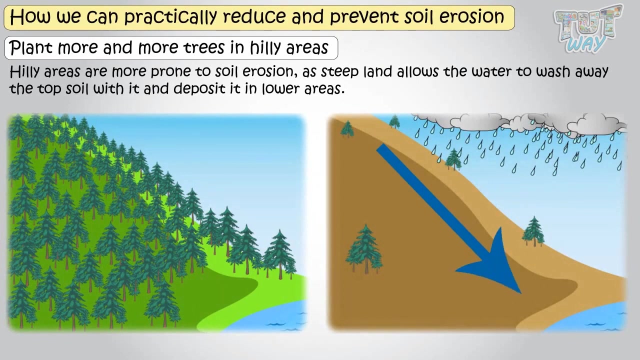 Plant more and more trees in hilly areas. In hilly areas, trees should not be cut, as tree roots hold the soil firmly and prevent soil erosion and landslides. Hilly areas are more prone to soil erosion as steep land allows the water to wash away topsoil with it and deposit in lower areas. 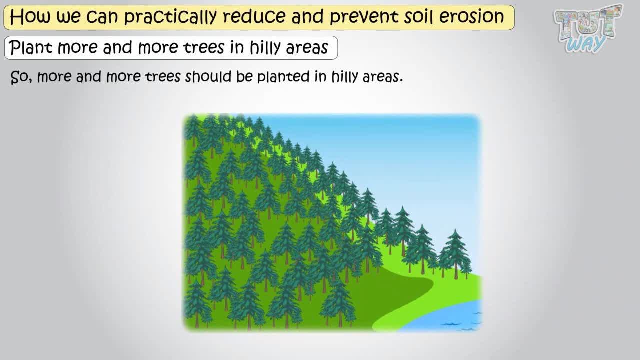 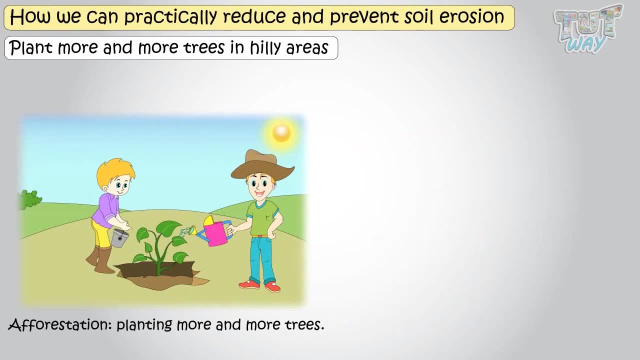 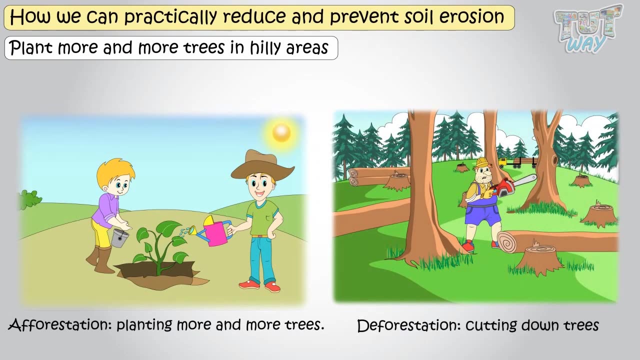 So more and more trees should be planted in hilly areas. Kids, afforestation means planting more and more trees, and deforestation means cutting down trees. Now let's learn another method to prevent soil erosion. It is reduced tillage. 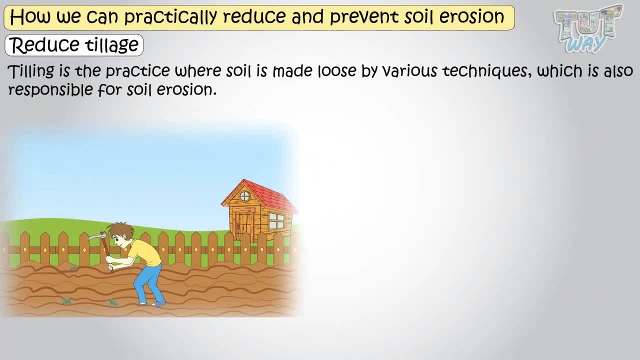 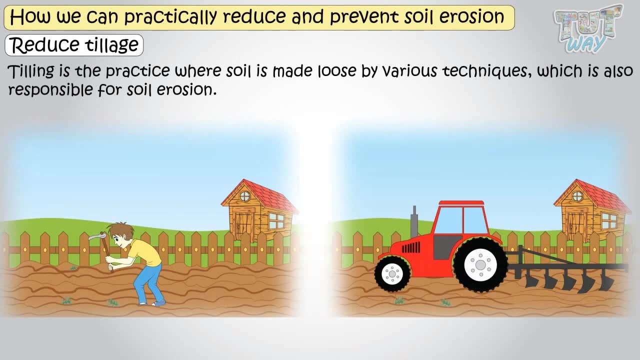 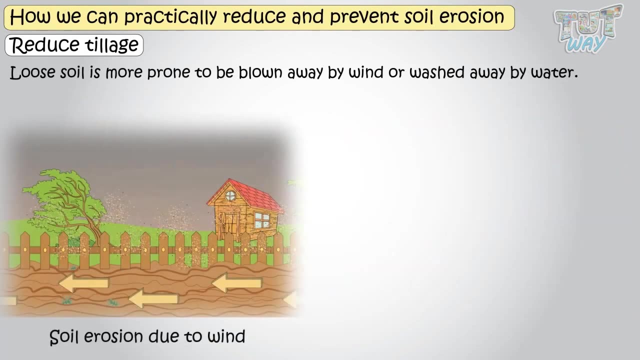 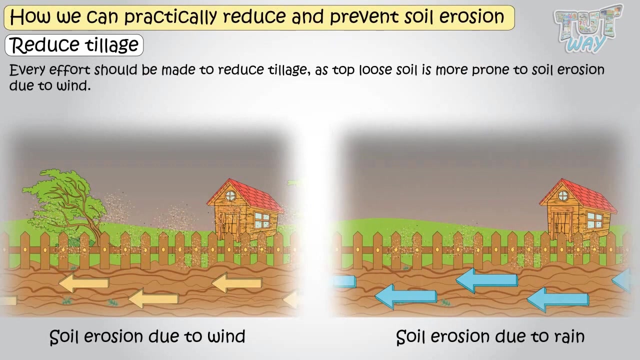 Tilling is a practice where soil is made loose by various techniques. That is also responsible for soil erosion, as loose soil is more prone to be blown away by the wind or washed away by water. Every effort should be made to reduce tillage, as top loose soil is more prone to soil erosion due to wind.